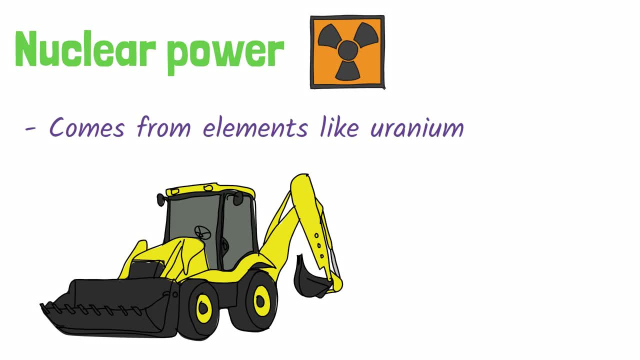 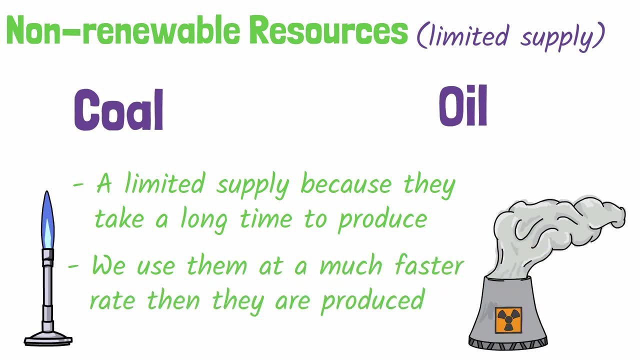 comes from elements like uranium that are mined from the earth. Again, there is a limited supply of all of these non-renewable resources because we use them at a much faster rate than they are produced. These resources are converted to power through the use of power plants, often to create 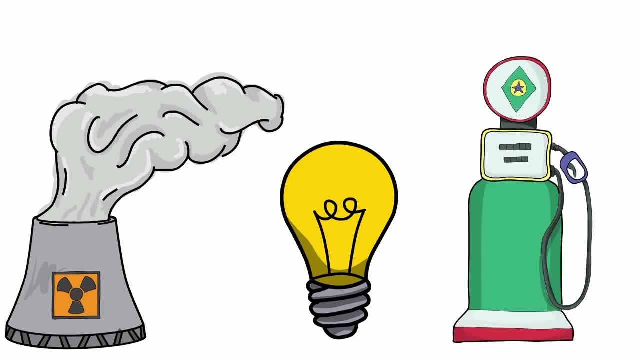 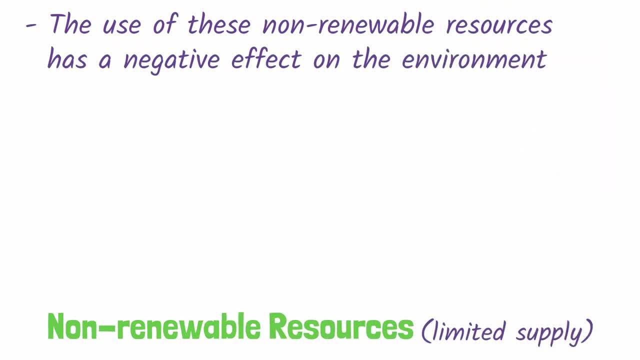 electricity or, in the case of oil, to fuel transportation. As you are likely aware, the use of these non-renewable resources also has a negative effect on the environment. This effect is large with reasons. For example, the use of non-renewable resources in the environment is: 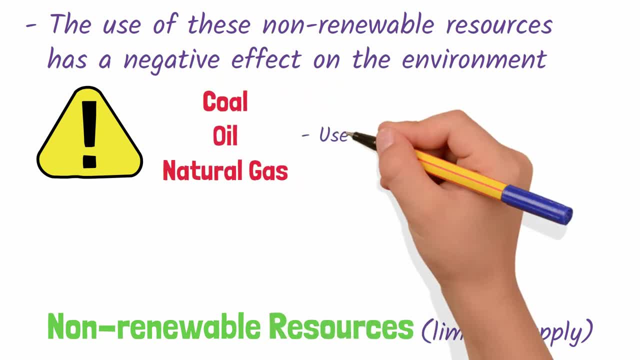 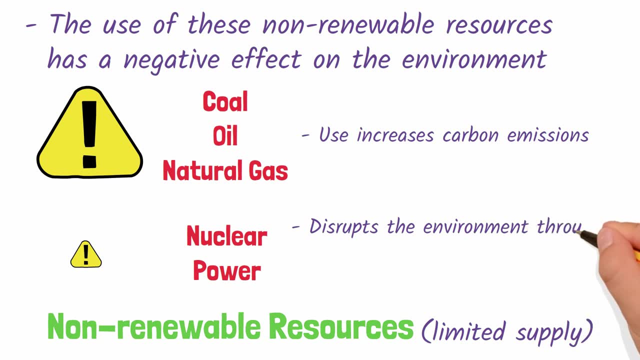 less effective than the use of natural resources like coal, oil and natural gas, the use of which increases carbon emissions. The effect is smaller with nuclear power, which primarily disrupts the environment through mining efforts and disposal of nuclear waste. Renewable resources, on the other. 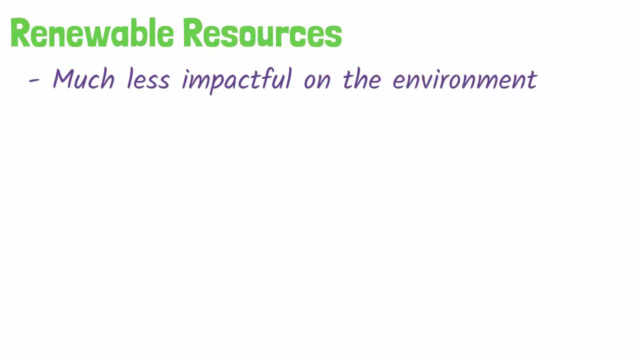 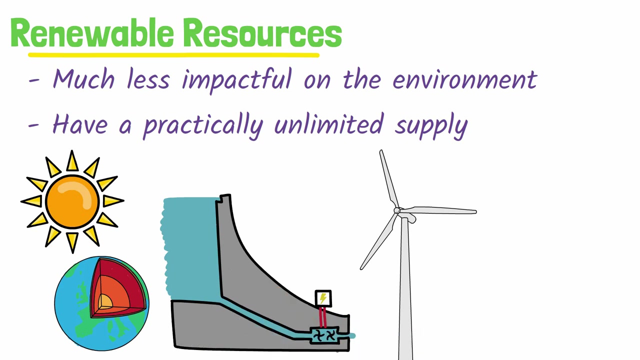 hand, are much less impactful on the environment. They also have a practically unlimited supply. That is why we call them renewable resources. These include solar power, wind power, geothermal energy, hydropower and biomass, which is energy from organic materials like wood and biofuels like 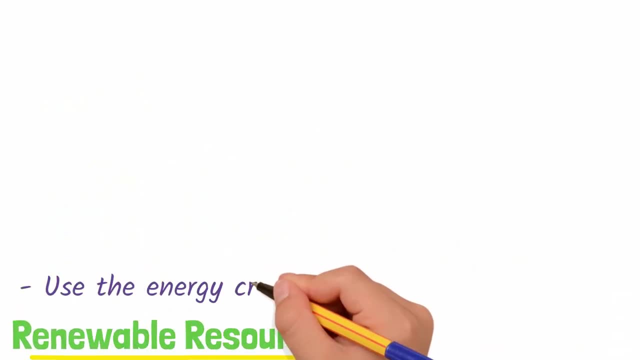 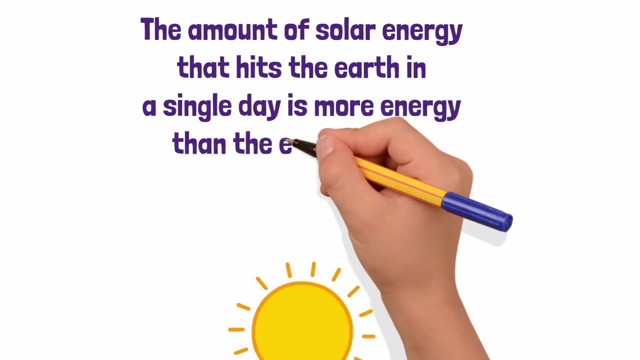 ethanol. Renewable resources use the energy created by nature on a recurring basis. The sun shining, the wind blowing and water flowing are all natural resources of energy for us to tap into. For example, the amount of solar energy that hits the earth in a single day is more energy than the 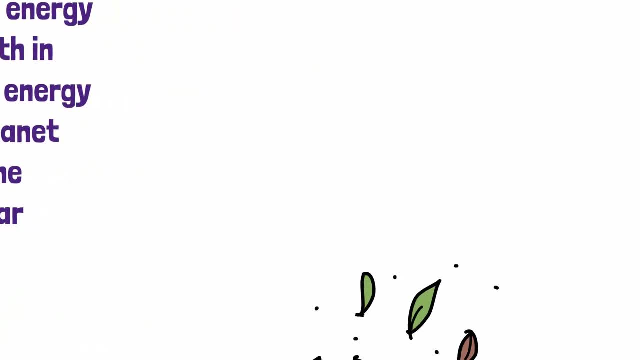 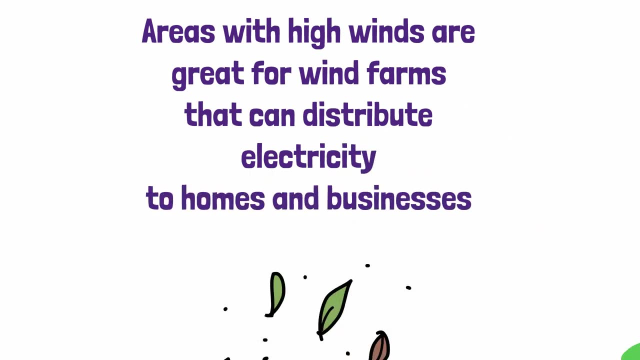 entire planet consumes in the course of a year. Areas with high wind and wind energy are more energy-intensive than areas with high wind. energy are great for groups of windmills called wind farms, which send energy to transmission stations to be distributed as electricity to homes and businesses. 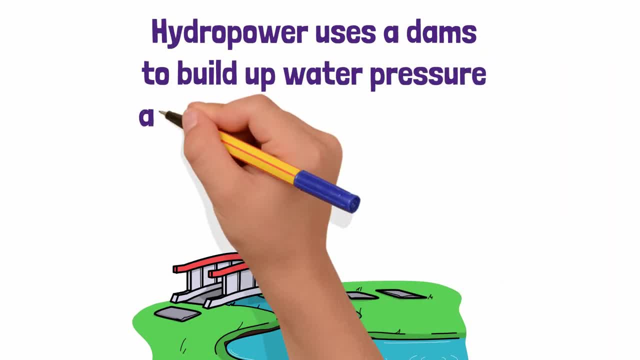 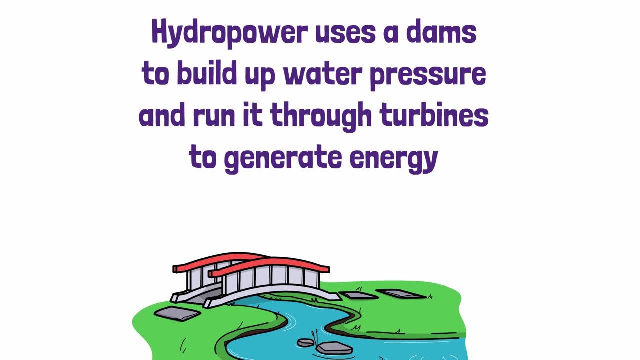 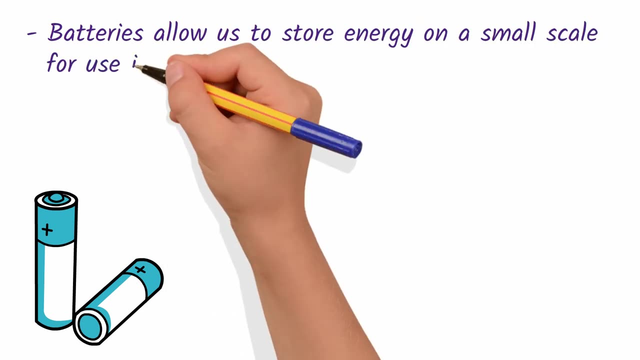 Hydropower works much the same way, usually using a dam to build up water pressure and run it through turbines to generate energy that is also sent to the transmission stations. Another big component of renewable energy are batteries. Batteries allow us to store energy on a small scale for use in our 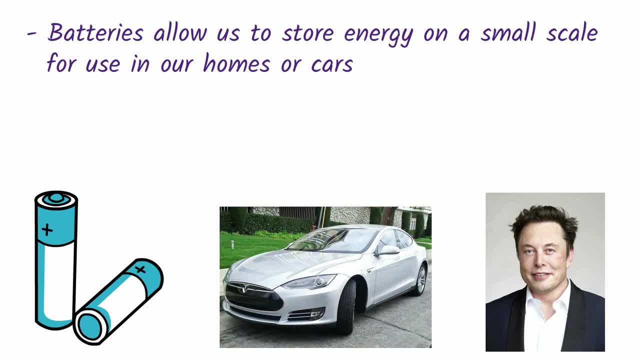 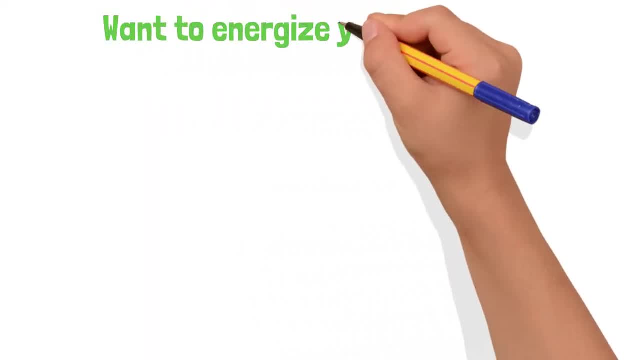 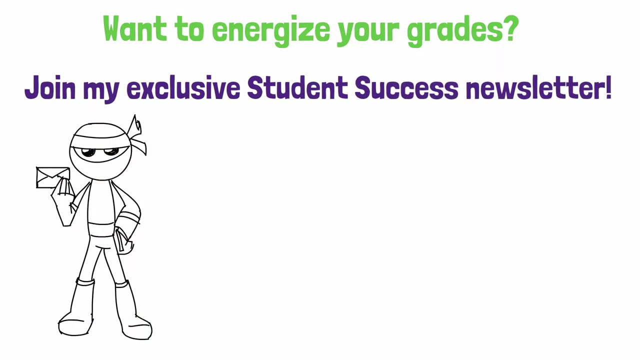 homes or cars, and this is how Elon Musk Tesla cars work. The better batteries we have, the more efficiently we can utilize renewable resources. If you want to energize your grades, then join my exclusive student success newsletter. You'll get quality tips in your inbox every month to help you succeed in. 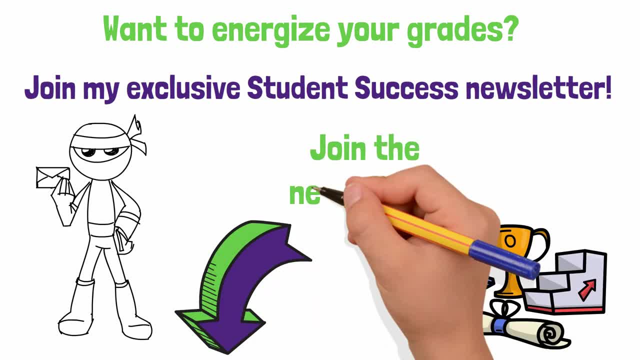 school and in life. Follow the link in the description to join the newsletter for free. Thanks for watching and I'll catch you next time. you.